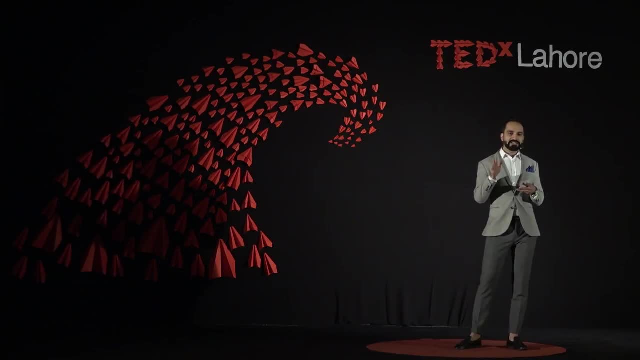 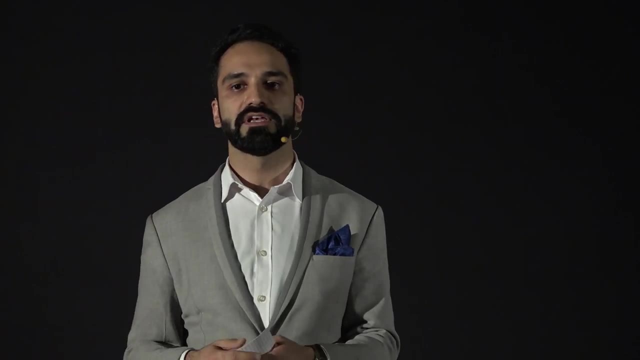 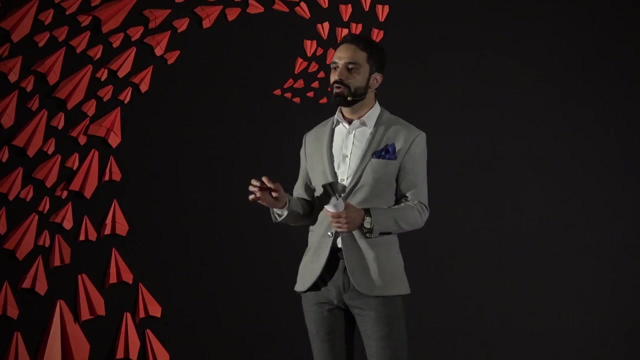 Now, what does this really highlight? and what did this really highlight at that time in our society, amongst our students? It was this acute and conspicuous lack of civic education at our educational institutions. We are never taught how our government works. we are never taught how our 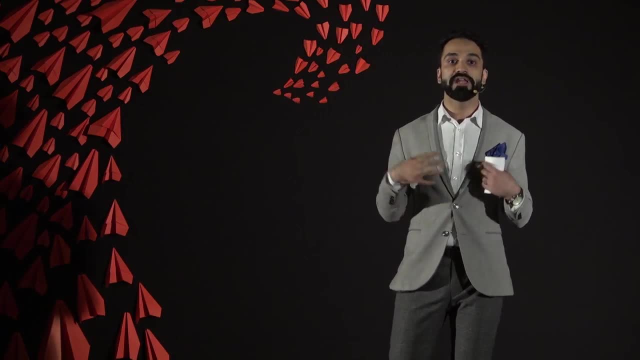 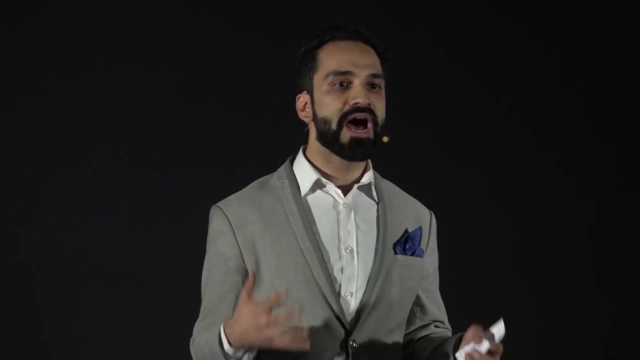 country functions and we are never taught what the laws are, and we are never taught what the laws are, and we are never taught what the laws are and how we, as citizens, can use them, And that is why I personally believe that civic education should be a mandatory subject. 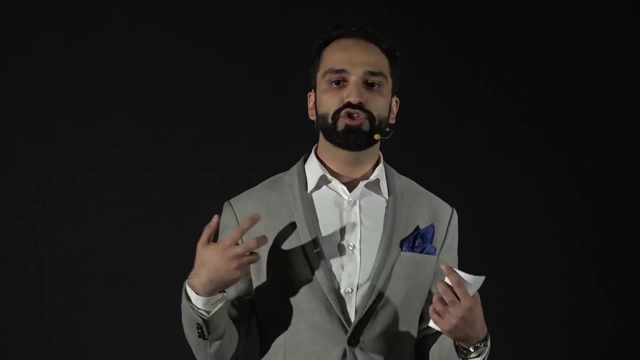 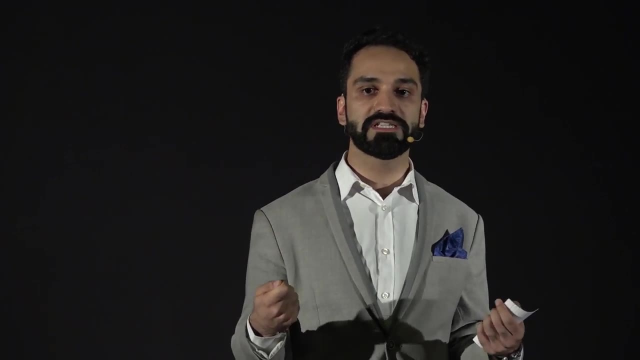 in all educational institutes in Pakistan that all students should learn what are their rights and they should learn how to file their taxes. they should learn how to file an FIR and how to deal with police when they're stopped, and they should learn how elections and how governments work. 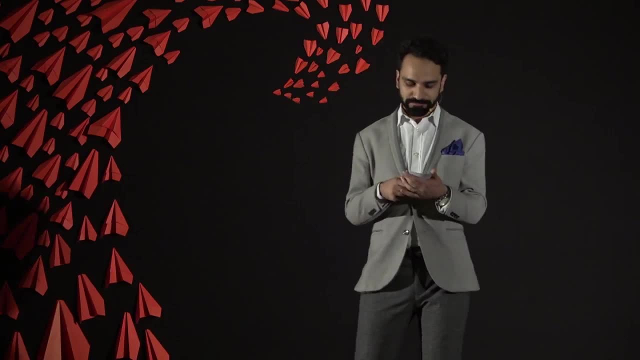 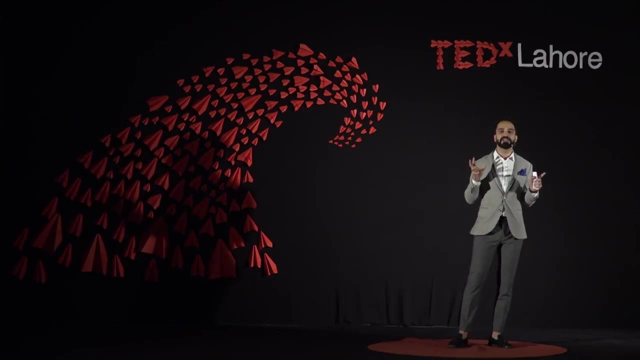 and how they can hold government officials accountable. Now, why is this important? Why is it important to hold government officials accountable And why is it important to push the system that we live in of politics, of government, of things we hear about in the news all the time? 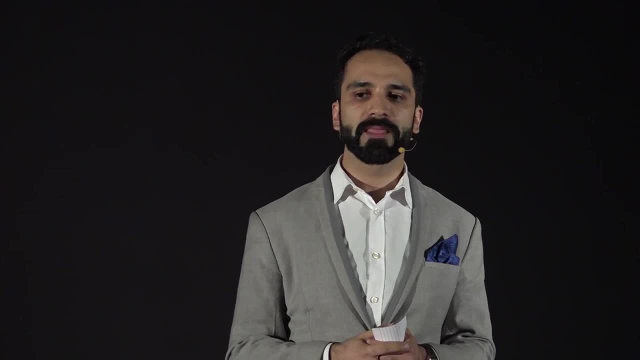 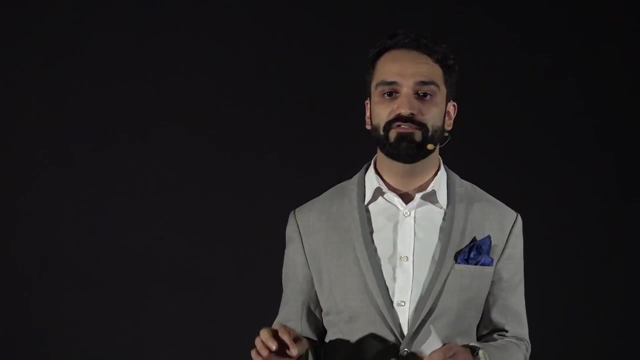 Why is it important for us to be involved in this? There are two reasons why it's important to be involved in this. First of all, it is your money, it is our money that is running the government, So it is through our taxes. 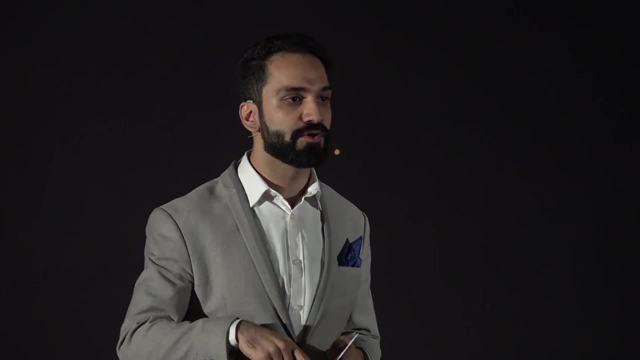 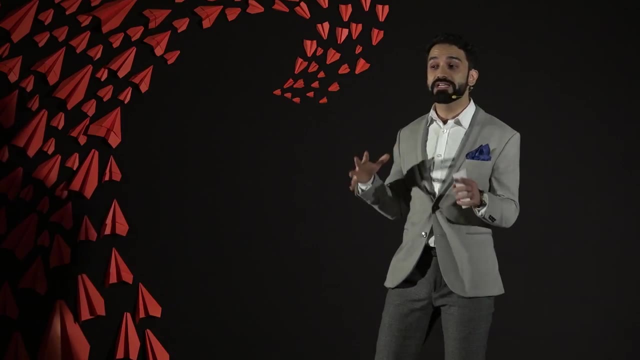 whether it's the 25% tax we pay on each mobile phone upload, or whether it's the income tax that's slashed off our incomes every month, off our salaries. that is what is running the government. that is what is paying the salaries of your policemen. 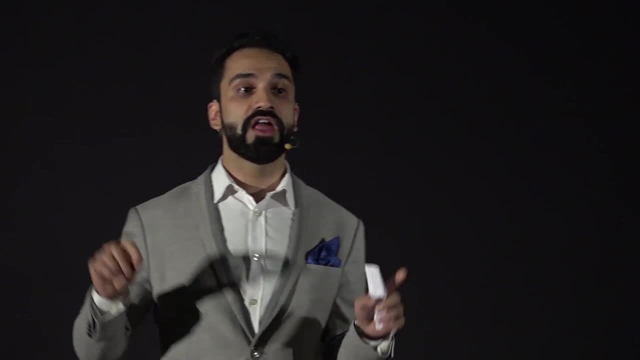 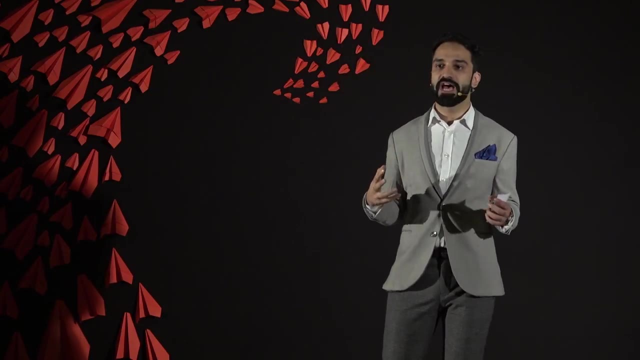 of your politicians, of your judges, of your generals and of everyone that works as part of the state institutions. And the second reason: it's important for us to be involved and it is important for us to hold our politicians and our state accountable. 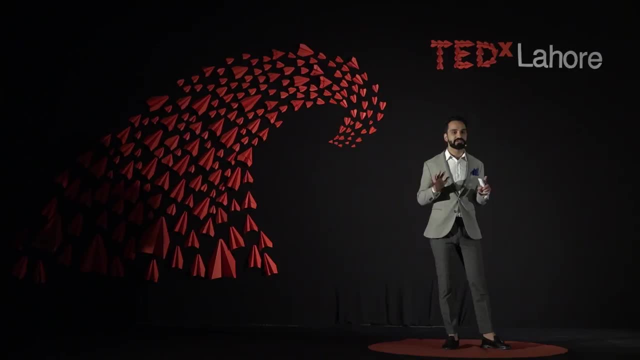 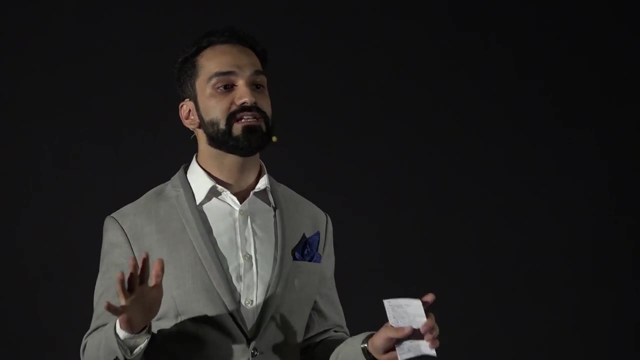 is because it is through our votes that our government really comes to power. So it's by virtue of our taxes that we're paying and of our votes that we're giving that the government really is able to perform. the government is really able to exert the power they do over us. 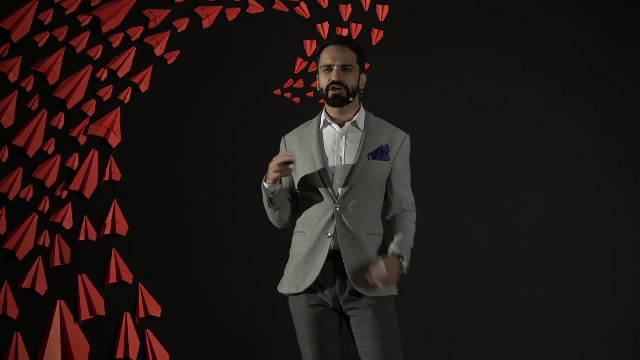 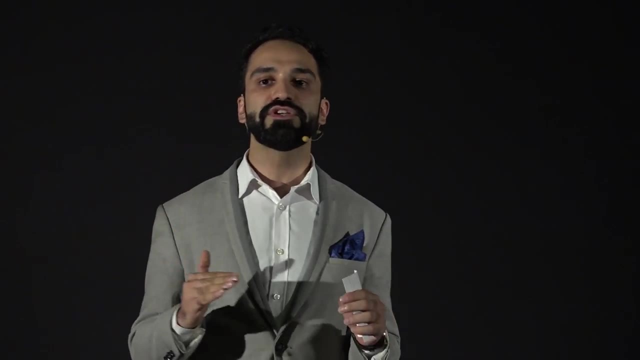 Now, the issue with this really is two-pronged. It's not only citizens that are not active and are not demanding their rights, but it's also the government and the state machinery that is not really equipped or is not really used to, you know. 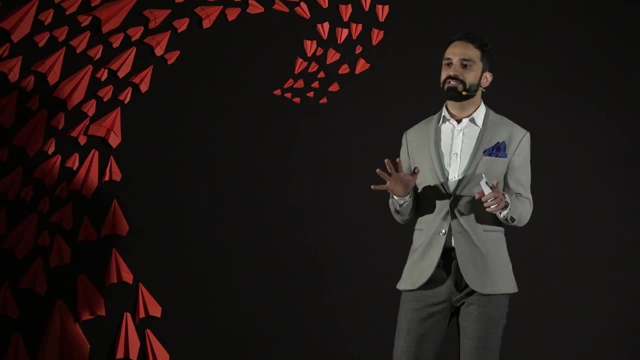 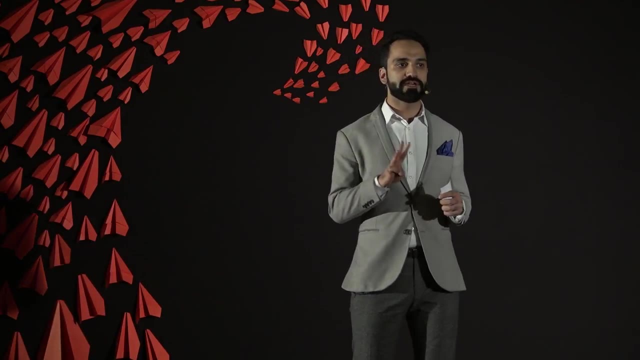 being accountable to citizens. I'll give you an anecdote, an example of what I've personally experienced. So in 2014,, I filed around three right to information requests with one government authority and with one ministry. Now there's a stipulated time under law of 21 days. 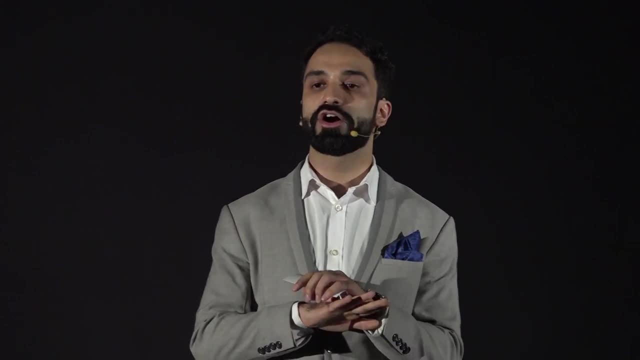 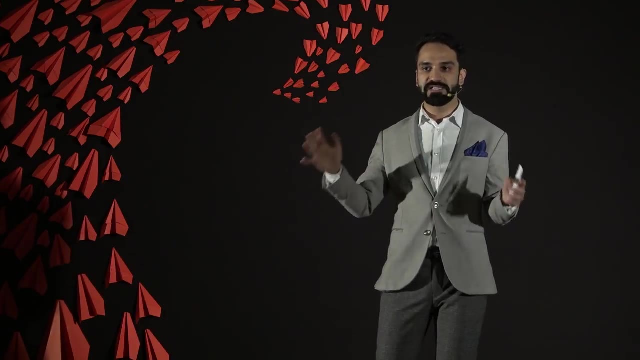 for them to give a response to your information request. I got no response, So then the procedure back then was that you appeal to the federal ombudsman office and that's senior retired government officials that then call a hearing between you, the citizen. 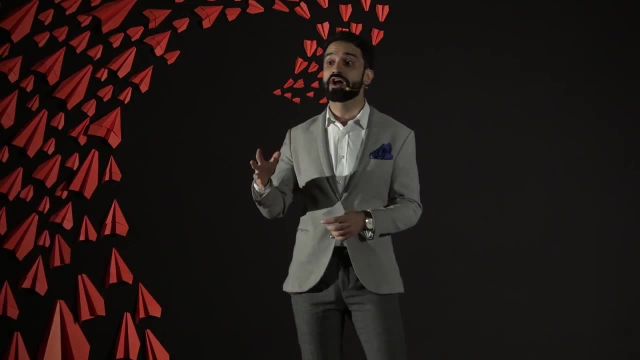 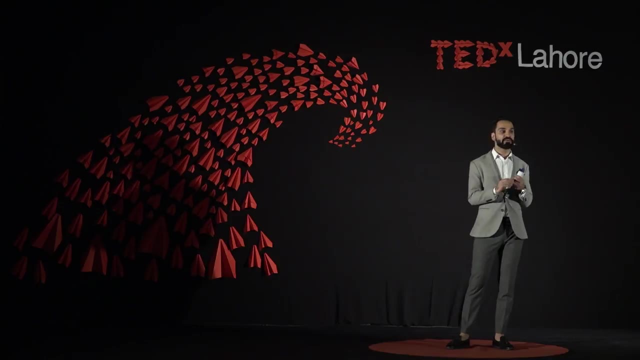 and between the officials from the government department that did not respond to your request. Now we sit at the hearing and this is 2014,- and we find out from the officer from the government ministry that in the 12 years since that freedom of information ordinance, 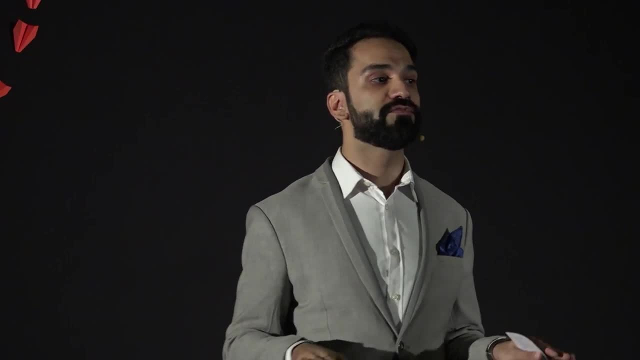 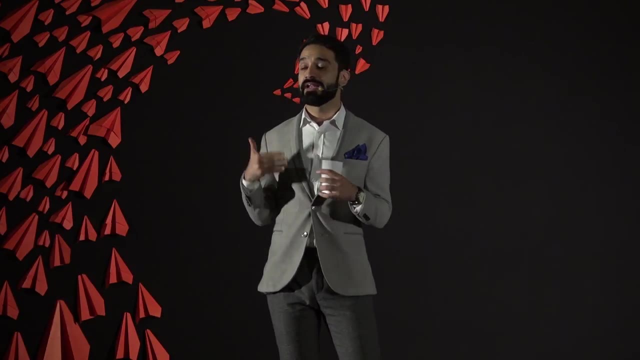 was promulgated. in that 12 years, they had never received a right to information request and they did not know what a right to information request was. Now, what happens next is very interesting and it will explain a lot of what I talked about earlier. 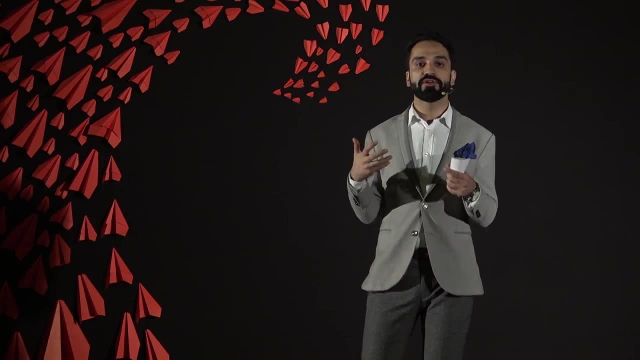 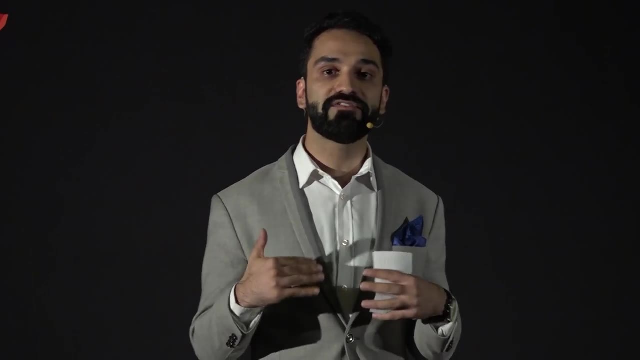 So our request was about the legal procedure for how the government is censoring websites in Pakistan. Back then, YouTube was still blocked and my friends in my organization we were very, very angry about how we could not access so many websites in Pakistan without any knowledge. 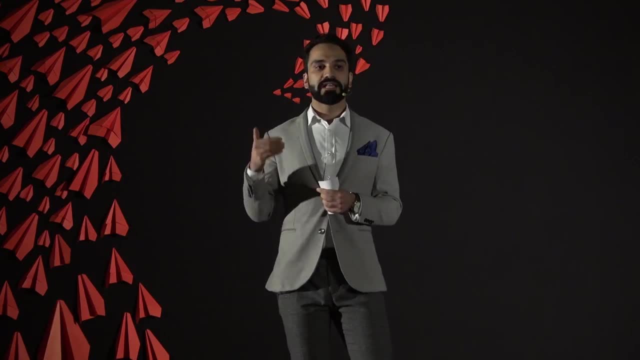 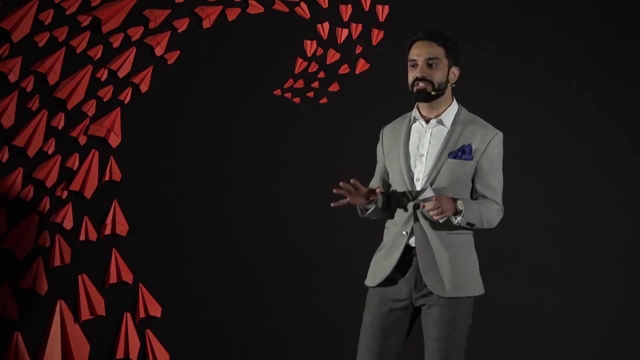 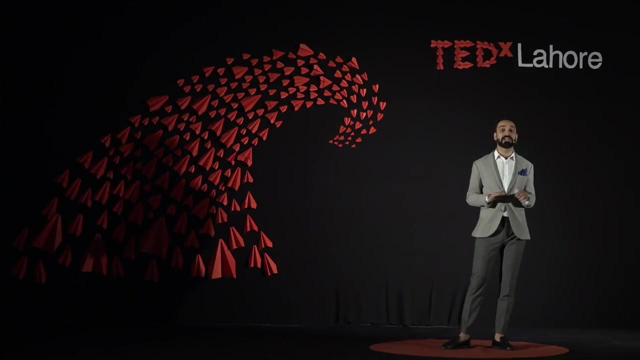 of why they were blocked. So we find out that in 2006,, an inter-ministerial committee for evaluation of websites was formed, and what that committee was doing was censoring all the websites that were being censored in Pakistan. However, before this, nobody knew about this committee. 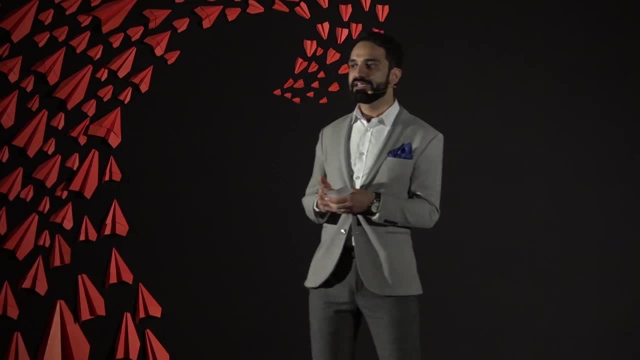 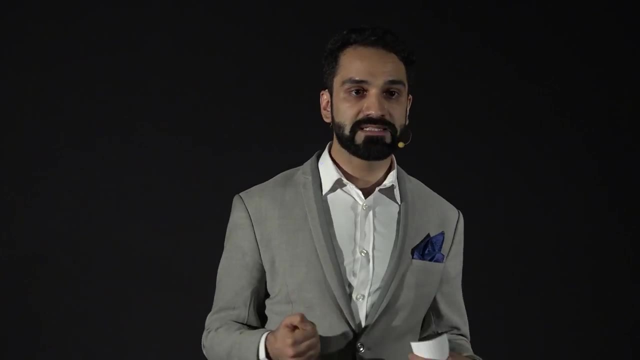 and it was not public knowledge. What we then realized is that this inter-ministerial committee is actually unconstitutional and it is not legal for it to exist. So my organization, BoloBhi- we challenged the inter-ministerial committee's existence in the high court. 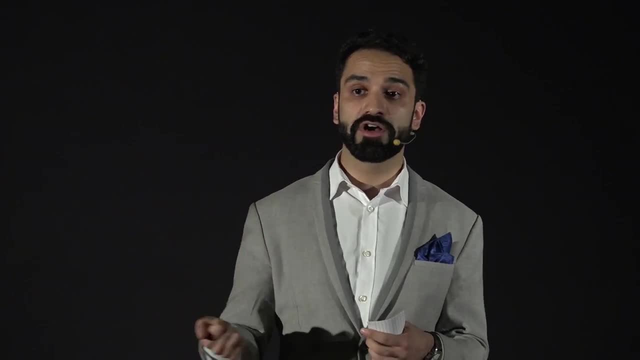 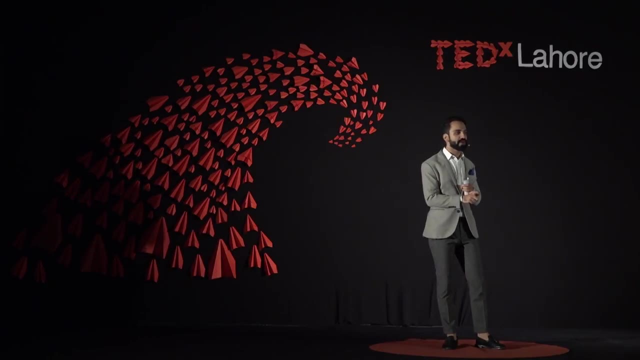 and what happened then was that the court ordered that it was actually unconstitutional and that committee was disbanded. Now, what does this show? Here's what it was. Had I not filed that right to information request, we as citizens would never know that this committee existed. 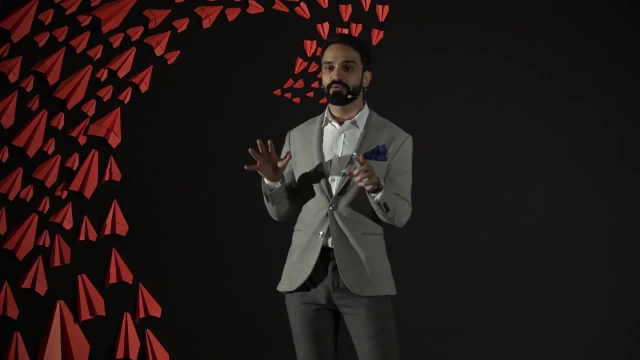 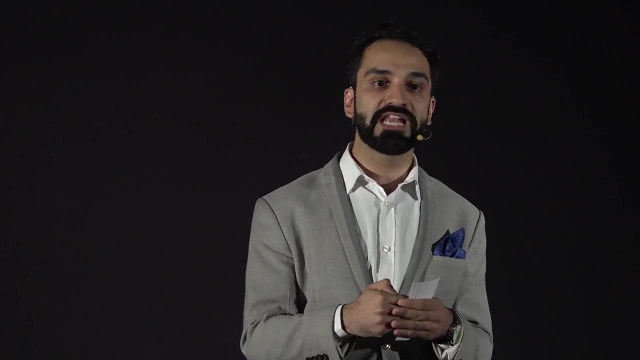 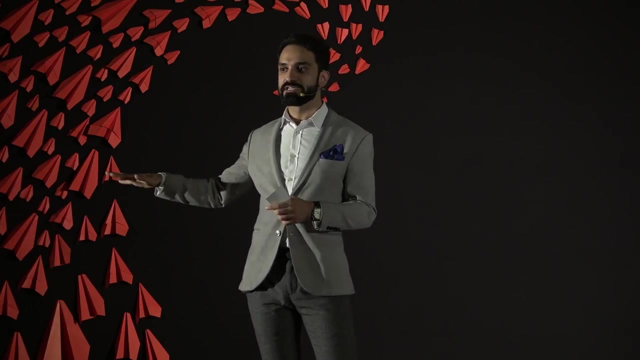 and would never know that this committee was unconstitutionally censoring websites on Pakistani internet. But once we had that information, we used the legal route of the court to challenge that and we got a favorable response from the court on this. So if citizens are ignorant, 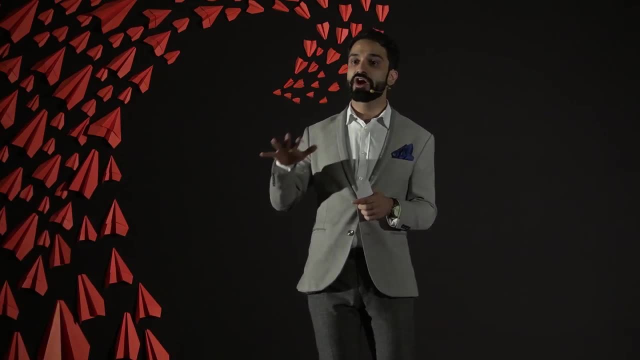 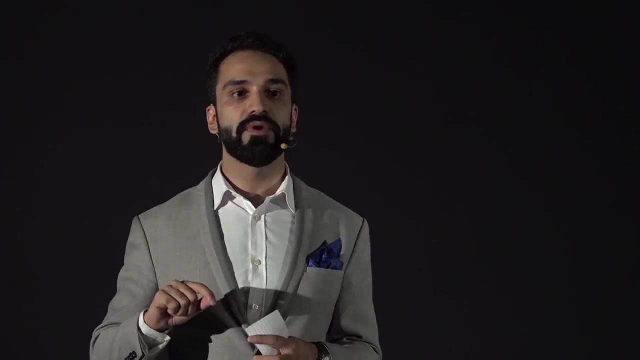 and if citizens are not holding the government to account, the citizens are not asking their officials what exactly they are doing. If citizens are not using the tools available to them in a democratic system, then the government and state officials will obviously abuse the power they have. 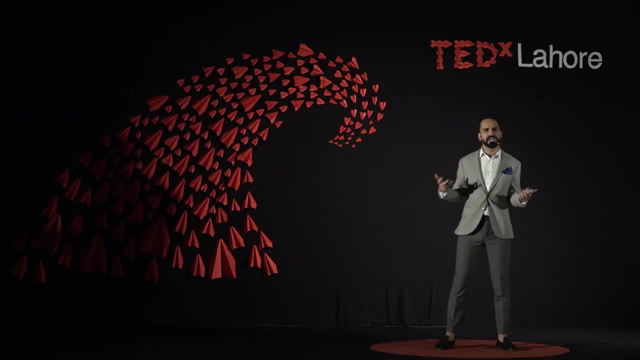 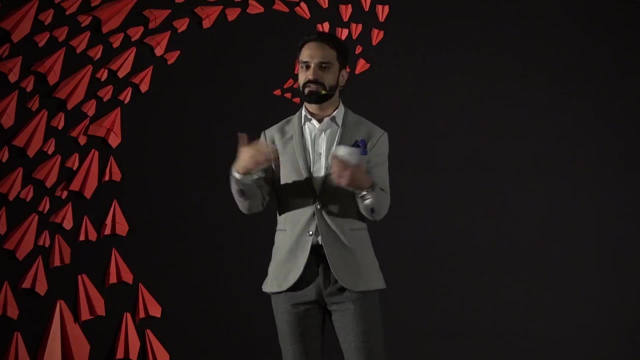 They will obviously be corrupt and they will obviously not have any interest in maintaining the government system the way it's supposed to go constitutionally. because the citizens do not know And because the citizens are ignorant, abuse of power is very, very easy. 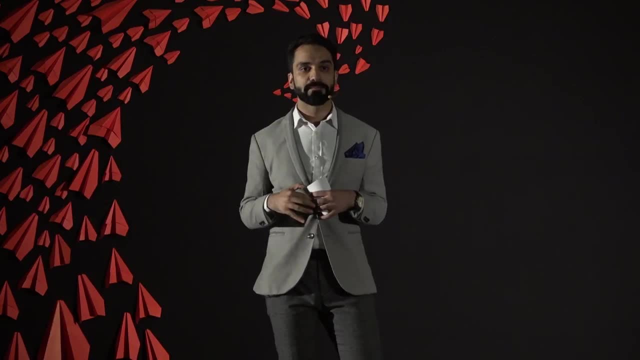 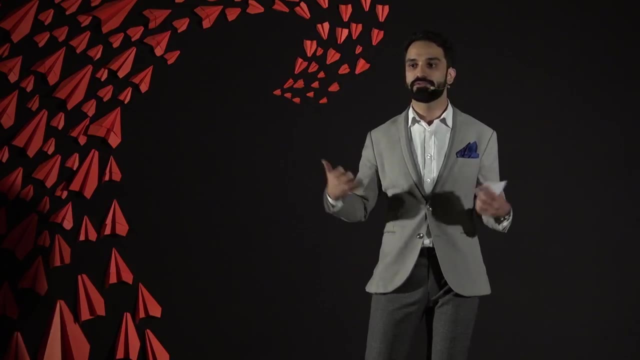 Now there's an explanation for this lack of democracy, the lack of democratic culture in Pakistan. If you look at our history, for hundreds of years we had monarchic rule. We had the Mughal dynasty and other dynasties who ruled over us. Until the fall of the Mughal dynasty. and then came British colonial rule. For 200 years we were a colony. We were under the British Raj and we were ruled by them Until 1947, when we finally got rid of the British. And then for the next 60 years. not a single civilian democratic government was able to complete its term, because it was interrupted by military coups and dictators. Now, the silver lining for us right here, right now is that the current government is the first that got power transferred. 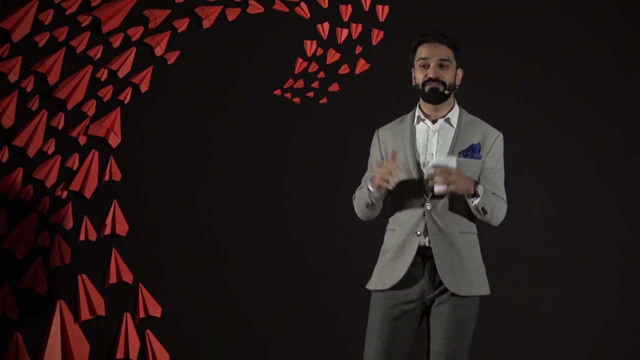 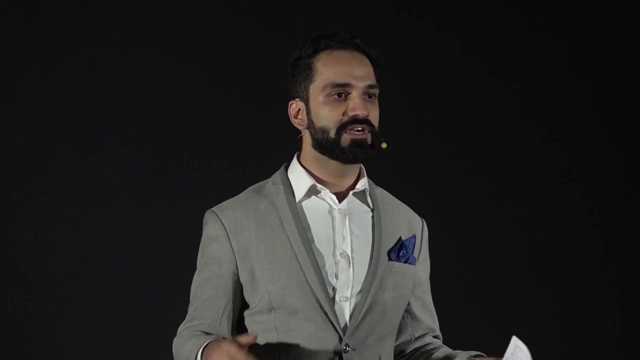 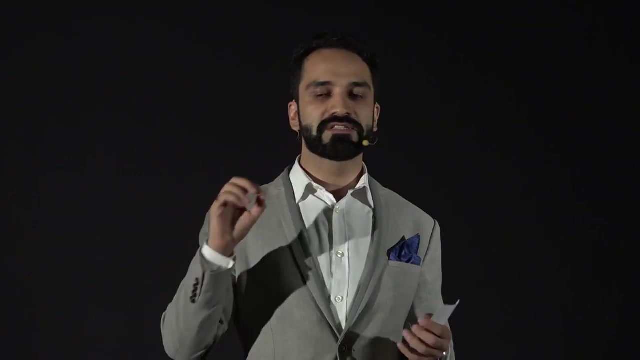 from another civilian, elected government. So we're a very young democracy and we're very new to this whole idea of us being the owners of this state, Because what's common across monarchies, across dictators and across colonial rule, It's the subjugation of people and the lack of accountability. 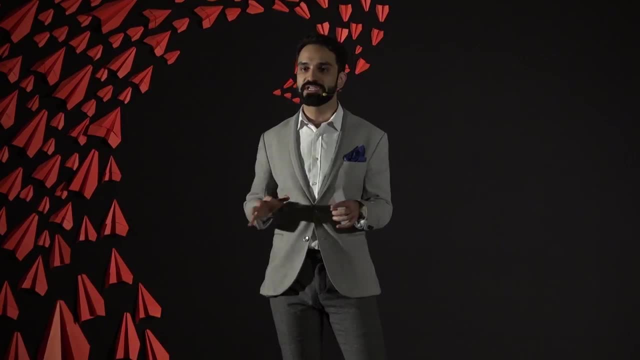 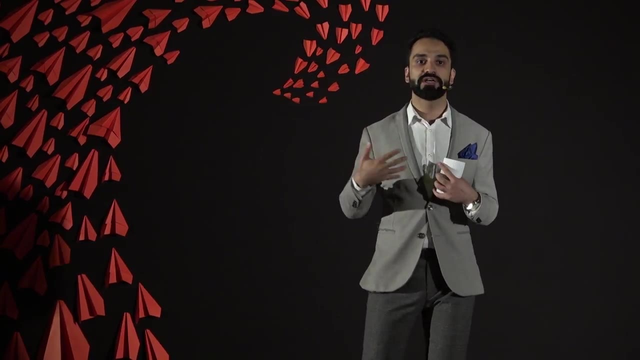 But now that we're a democratic country, now that we are voting, now that we have taxes and we have a system, it is our responsibility as citizens to demand greater accountability and to get rid of that culture where we have waderas and we have politicians thinking they own us. 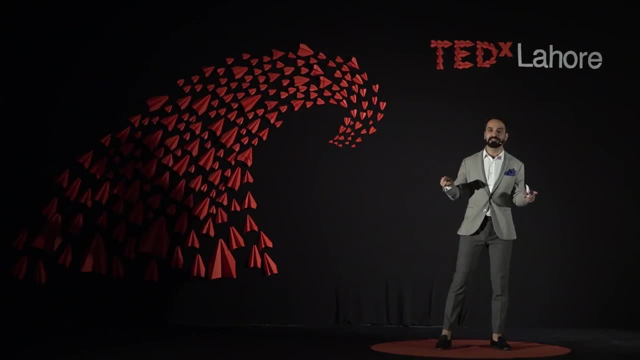 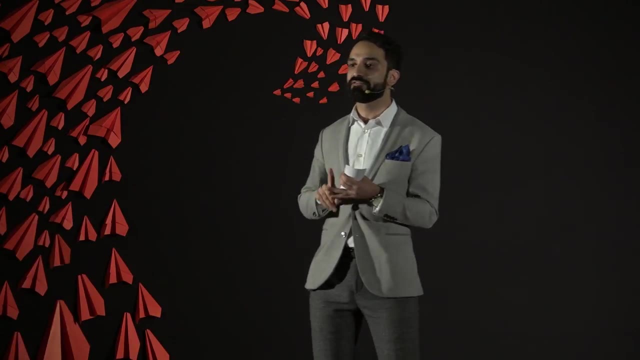 We own them, We pay them, We pay the taxes and we give them the votes. So we're entitled to every bit of good governance and every bit of our fundamental rights, as they're guaranteed in the constitution. So how is it that you and me, as citizens, 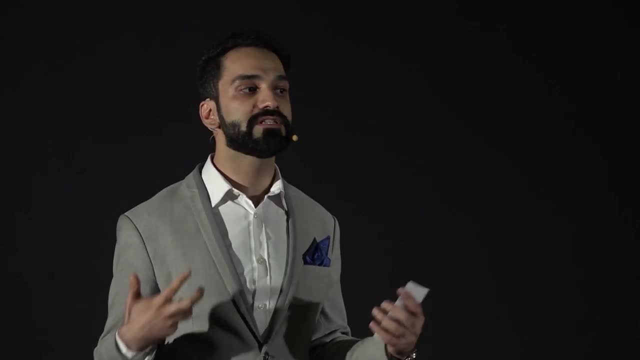 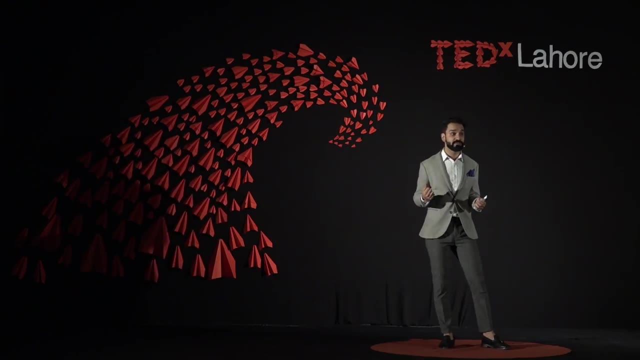 can really hold the government accountable and can really hold the state accountable and can really get them to run the country the way it's supposed to be run. So, first of all, I already talked about right to information requests, So any one of us can submit a right to information request. 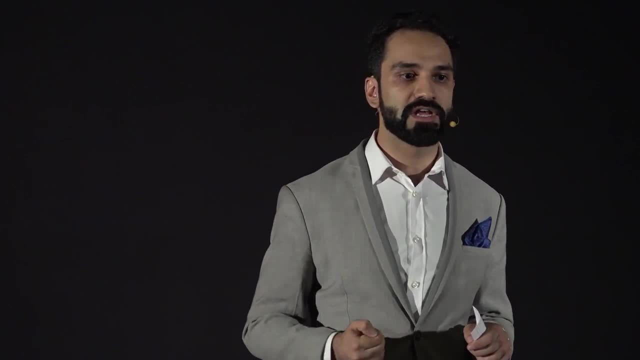 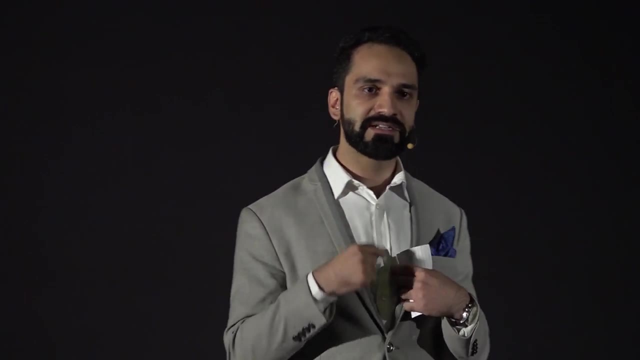 with the government department and demand information. And if you do not get the information, it's very fun going to the ombudsman and complaining and having a hearing and saying My taxes are your salary and I want to get this information. 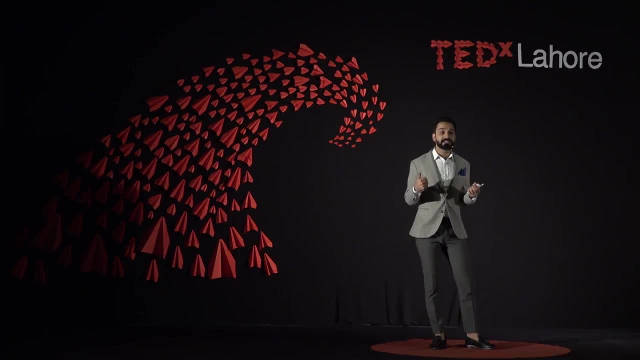 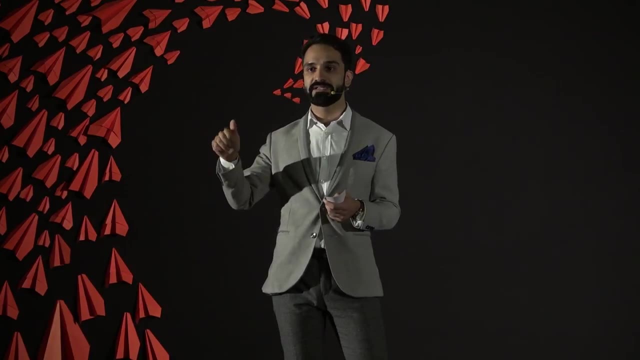 And I've done this. The second way you can do this is you can contact your representatives. I don't know how many of you knew this, but all the telephone numbers of your public representatives, of your members of provincial assembly, national assembly and senate, are on the website. 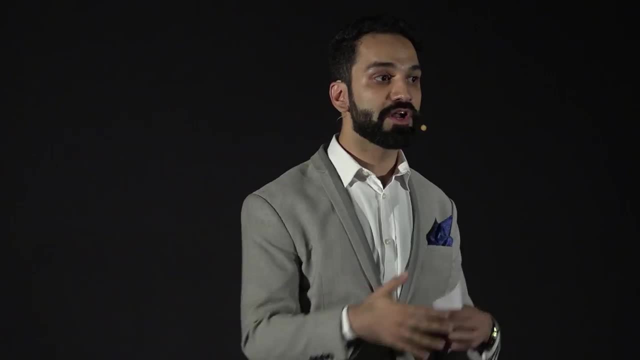 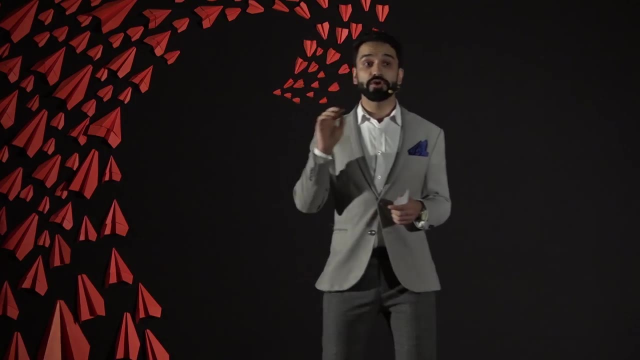 So if there's any policy or any law or any issue you're worried about in your area or overall, you can simply contact them through a text message or a phone call. You can also call any citizen of Pakistan. A citizen of Pakistan can call a public hearing in the parliament. 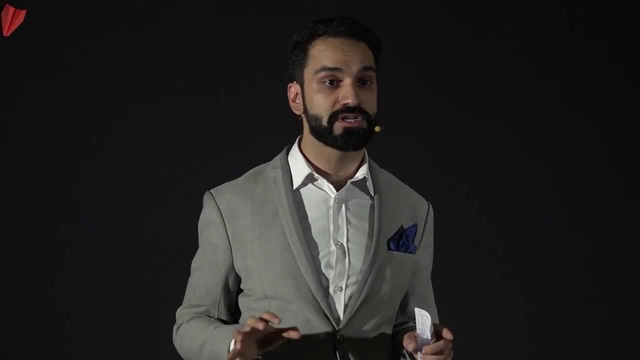 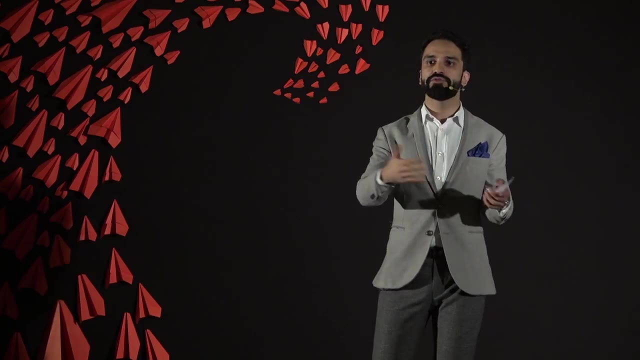 in the national assembly or the senate on any issue that you think is important, and they have to respond to you. So any of you can interact with them and ask them: Hey, why is this issue not being worked upon? Why is education in a mess? Et cetera, et cetera. 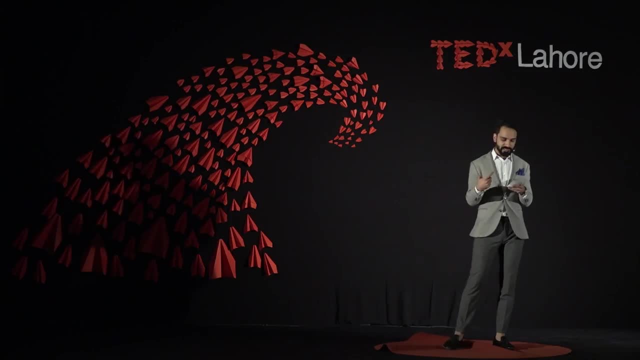 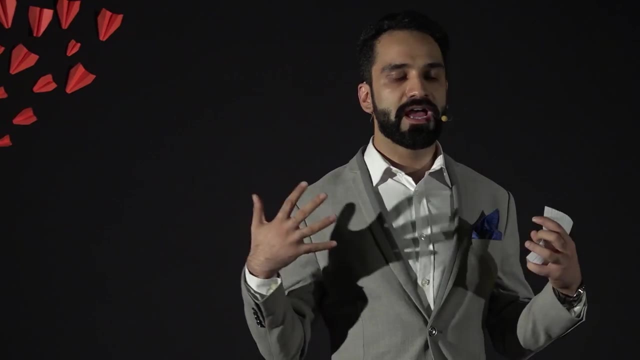 So there's a lot of different tools that are really available to us that we really need to start using Now. personally, when I realized the need for civic education when I applied for my master's, civic education was based on me wanting to come back. 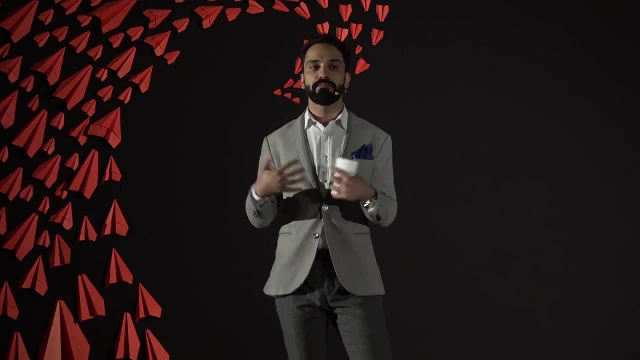 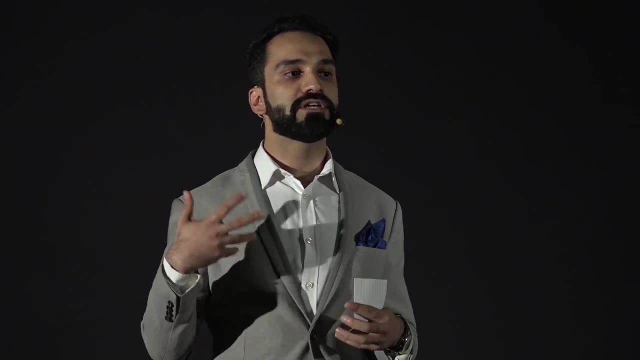 and to work on civic education. So when I came back, along with a few friends, I made a curriculum and we did a few trainings, But then, as mentioned earlier, I was able to really write a curriculum on fundamental rights in the Pakistani constitution. 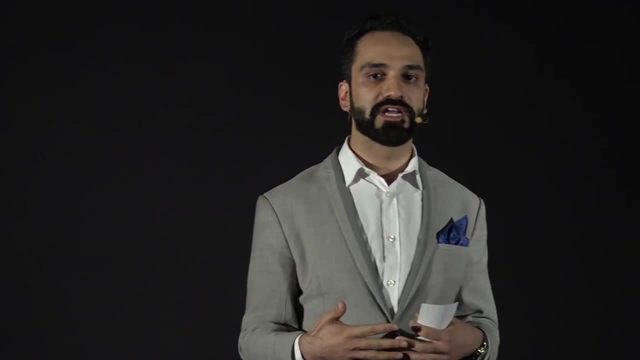 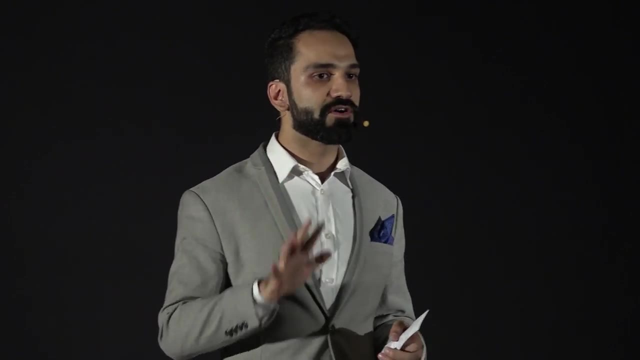 and that is now being tested at 11 universities in Pakistan as mandatory. And now, hopefully, if we keep trying to hold the government accountable, if we keep pushing for our rights to be known to us, if we keep pushing for a civic education curriculum,